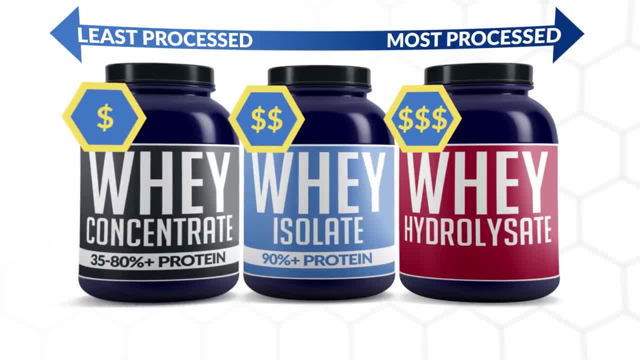 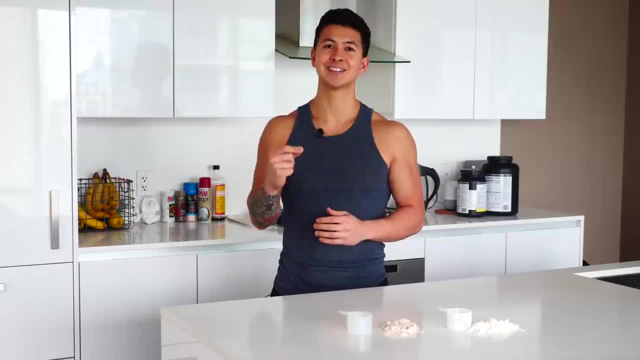 you first get well informed of the various differences between the various types of protein powders out there, as well as the things to look for and things to avoid when you compare different brands. By the end of this video, you'll know exactly what type of protein is right for you. 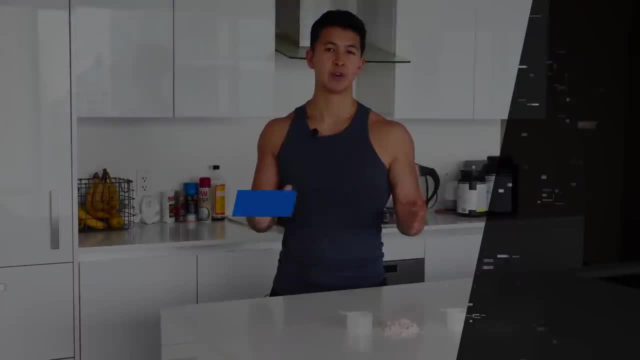 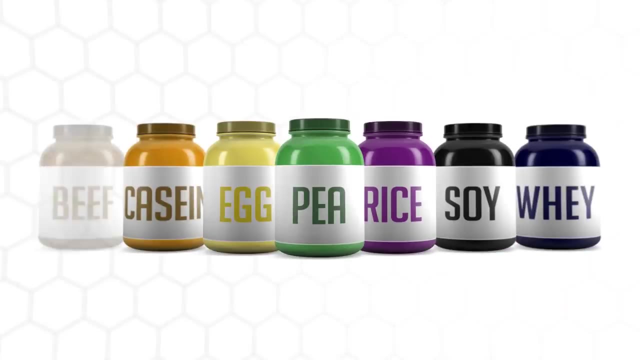 and how to separate the good from the not so good options out there. First, let's cover what type of protein powder may be best for you. Despite the overwhelming amount of different protein powders on the market, research has made it clear that whey protein comes out on top. This is because 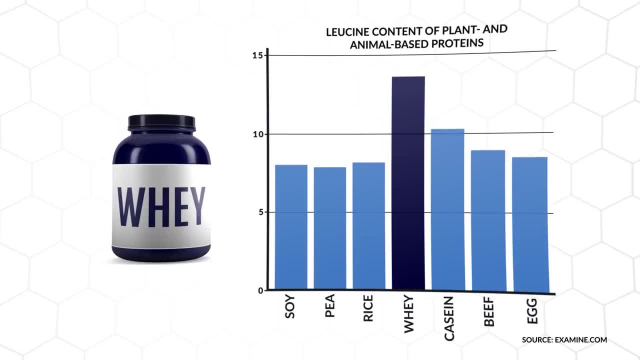 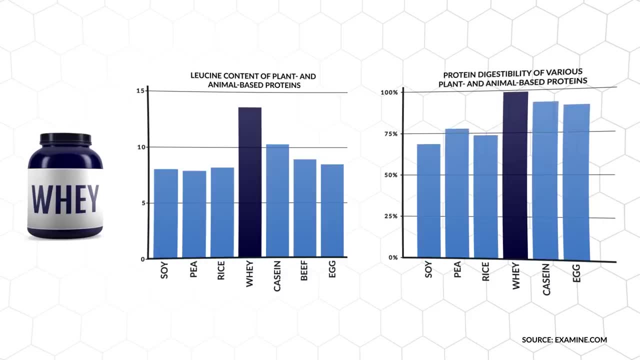 whey protein is both higher in leucine, one of the most important amino acids for muscle growth, and more effectively absorbed and used by the body when compared to various other protein powders and other protein sources. in general, Casein protein does come in. 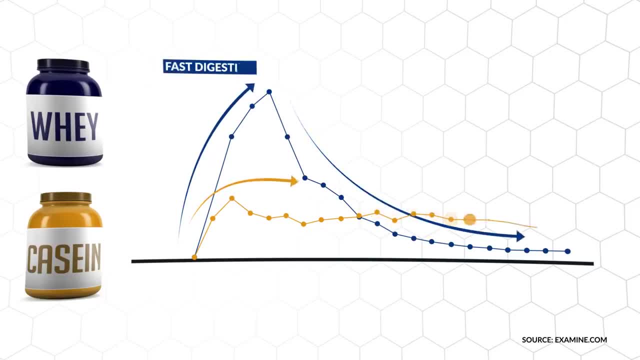 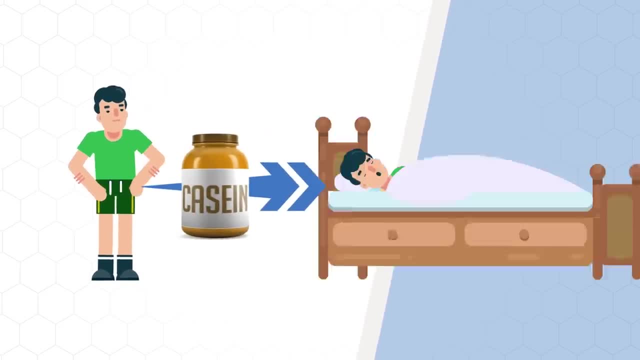 at a close second, with a slightly less leucine and overall protein content, but it is a much slower digesting protein than whey. In theory, this would mean that casein would be the more effective option to take as a pre-sleep meal so that we can stimulate. 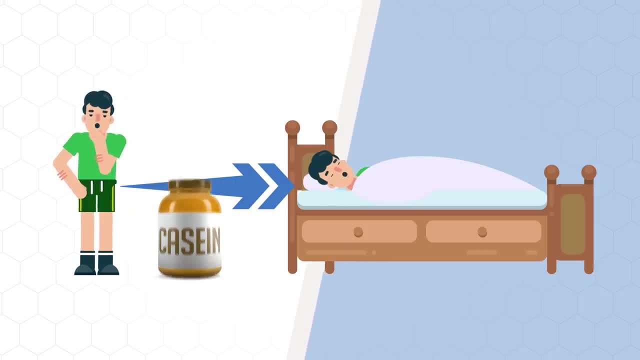 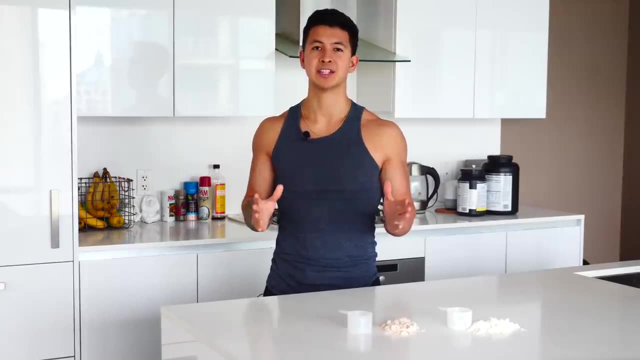 protein synthesis overnight. However, recent research seems to suggest that any high quality protein, such as whey, would do the job just as effectively, So whey seems to be the best option. but whey protein can be further broken down into three different types: Whey concentrate. 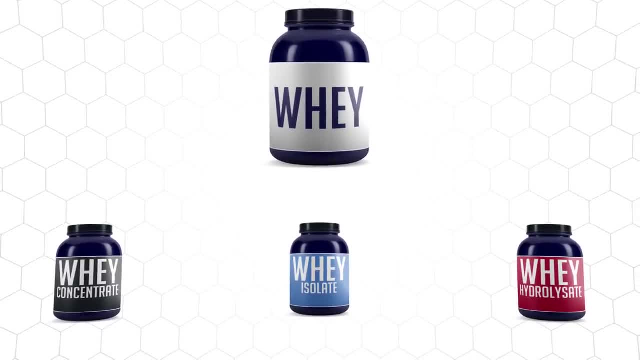 whey protein and whey protein. Whey protein can be further broken down into three different types: Whey concentrate, whey isolate and whey hydrolysate. The main differences here is that whey concentrate can range anywhere from 35 to 80% protein. 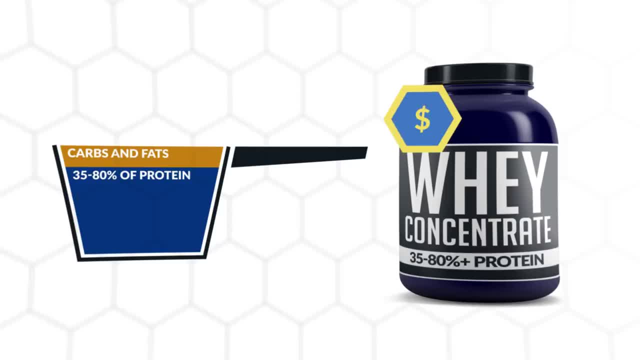 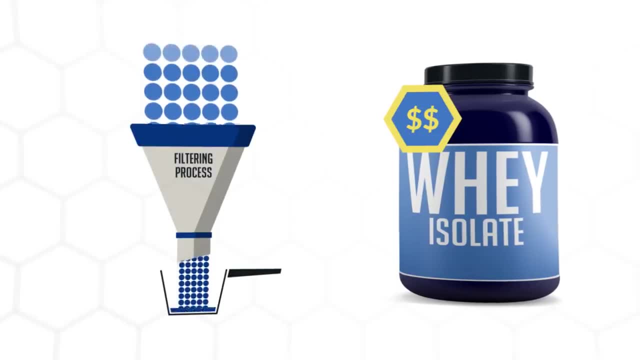 and typically contains the highest amount of lactose, carbs and fats, Whereas whey isolates, although typically a bit more costly, have to go through an additional filtration process and are required to be at least 90% protein by weight and therefore have considerably 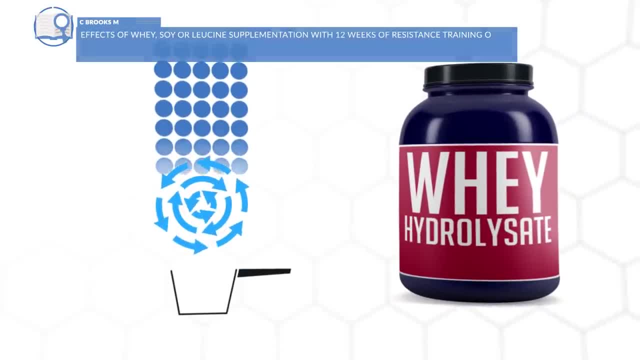 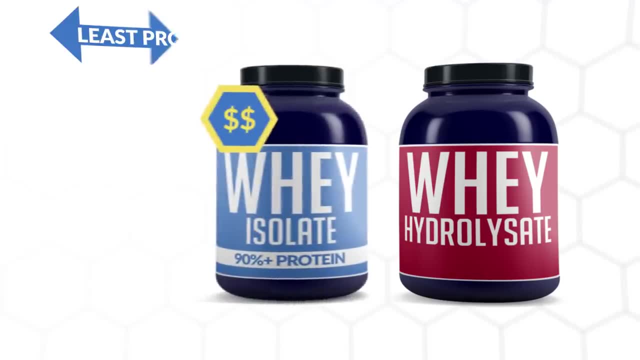 less fats and carbs. Hydrolysates, on the other hand, are whey concentrates or isolates that have just been pre-digested to help with its absorption, but have not been shown to be any more effective at increasing size or strength as the other two options. yet is typically the 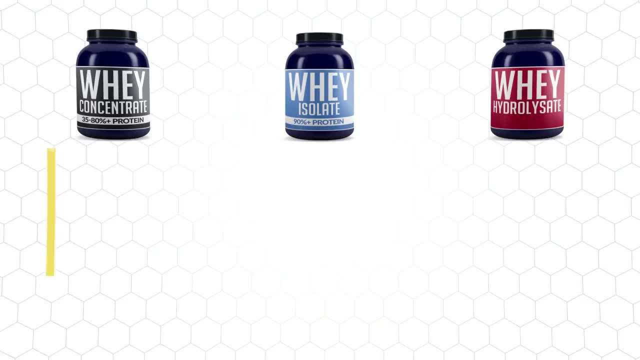 most expensive option, So essentially it's just like buying chicken. Whey concentrates can be thought of as chicken thighs- They deliver a good amount of protein but come with additional fat and calories, Whereas whey isolate can be thought of as chicken breasts, a bit more costly than 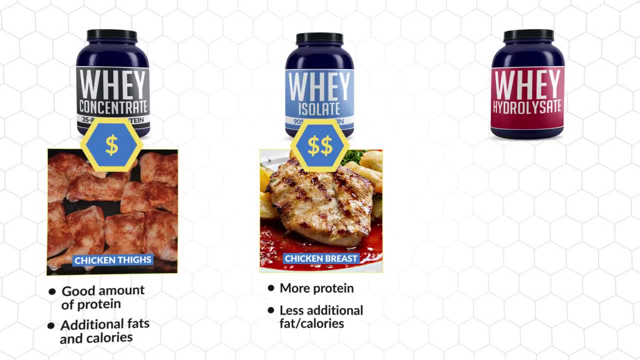 thighs, but pack a much higher protein content, with less additional fat and calories. Whereas whey hydrolysate could be thought of as extra lean ground chicken breasts, It goes through a bit more. processing is typically the most expensive option, yet it delivers the same amount of protein relative to calories, fats and carbs as chicken. 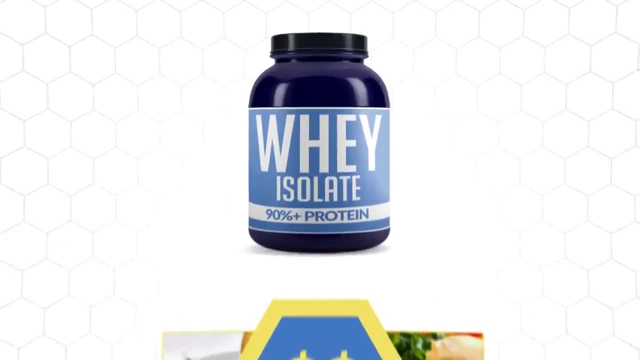 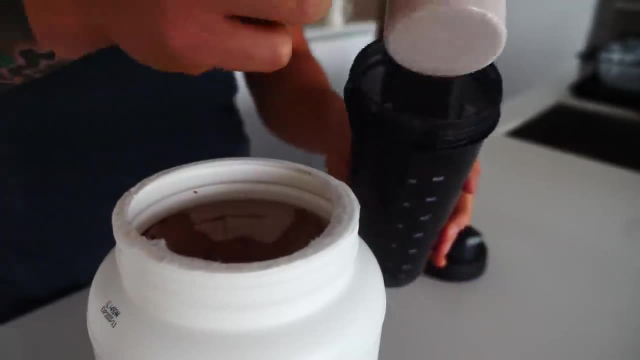 breast does, Meaning that for the best bang for your buck. for most people, a good quality whey isolate protein is your best bet, as it delivers the highest amount of protein and is slightly better for those who are lactose intolerant or just tend to have digestive issues in general. 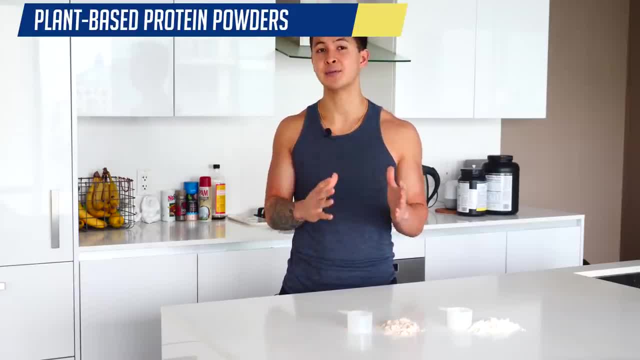 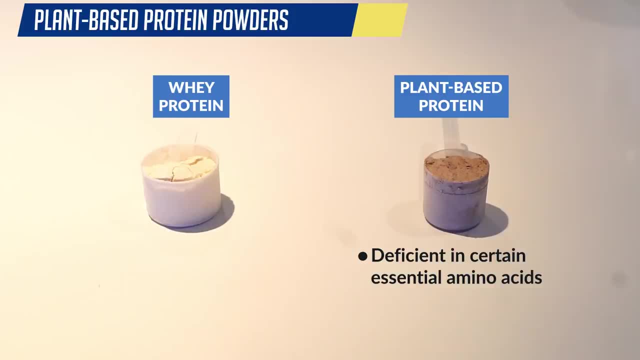 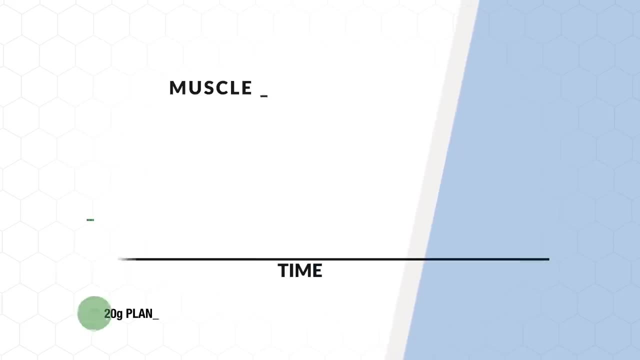 Now, as for plant-based options, this can be a good option if you do have intolerances or sensitivities to whey. The problem with plant-based proteins, though, is that they tend to be deficient in certain essential amino acids and are less effective at promoting protein synthesis than whey is, but research has shown that you can partially. 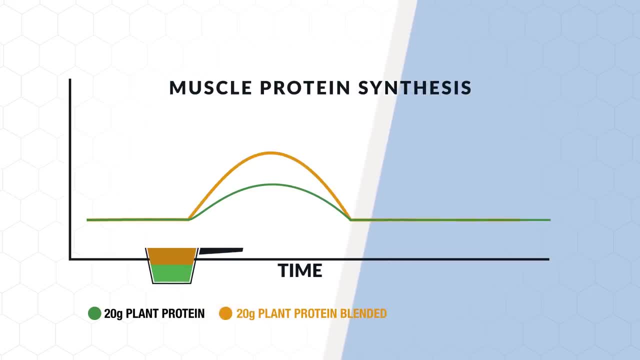 compensate for this by combining different plant-based protein sources. For example, pea protein is low in the essential amino acid methionine, whereas rice protein's low in amino acid methylane, and one recipe whey protein less volatile with. Those are some of the things that plant-based learn not to alter Arkans power and slightlyowego amiga protein s sources. For example, pea protein is low in the essential amino acid methionine, whereas rice protein is low in the essential amino acid methionine, whereas higherilia protein is low in essential amino acid methionine, whereas 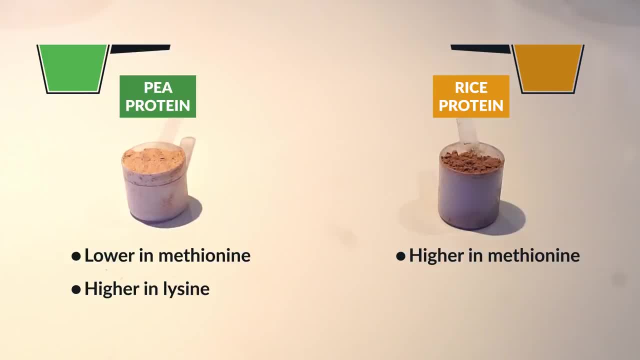 whereas rice protein contains considerably more methionine but is lower in the essential amino acid lysine, meaning that when you look for a plant-based protein powder, one with a good blend of rice and pea protein would likely be the best option. Soy protein, although subject to much controversy, is 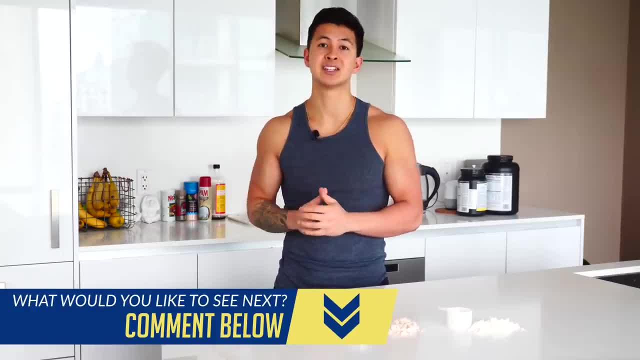 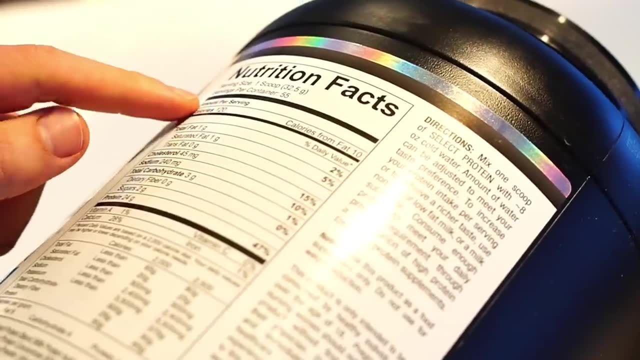 another good plant-based option, since it has a good amount of all the essential amino acids and is therefore something worth considering. Now, after you've chosen the protein powder that best suits your needs, the next step is learning how to separate the good brands from the not-so-good brands. 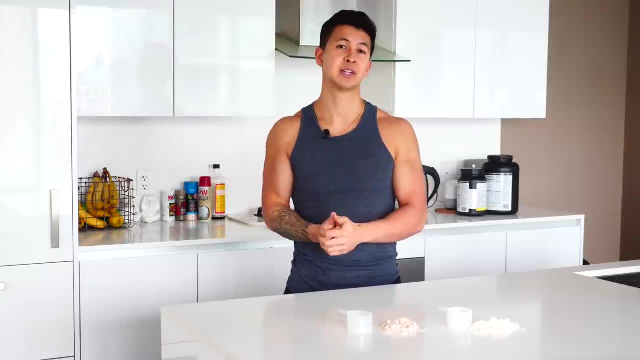 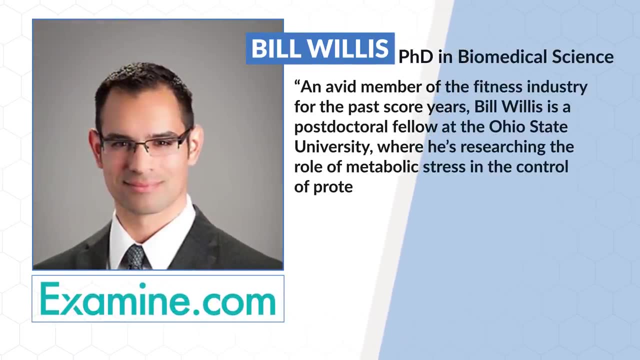 because, unfortunately, there's a lot of tricks that supplement companies can use to deceive you. And to help us out with this is Examinecom researcher Bill Willis, who has done a considerable amount of research and work within this exact topic. So, Bill, the first thing that you recommend that we look out for is the 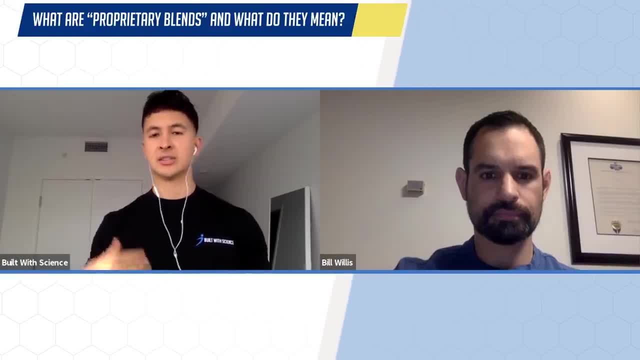 use of something that's called proprietary blends. Would you mind just explaining a little bit more about what exactly that is and then what that means for us as a consumer? So, Bill, the first thing that you'd recommend that we look out for is the use of something that's called proprietary blends. Would you mind just explaining a little bit more about what exactly that is and then what that means for us as a consumer? 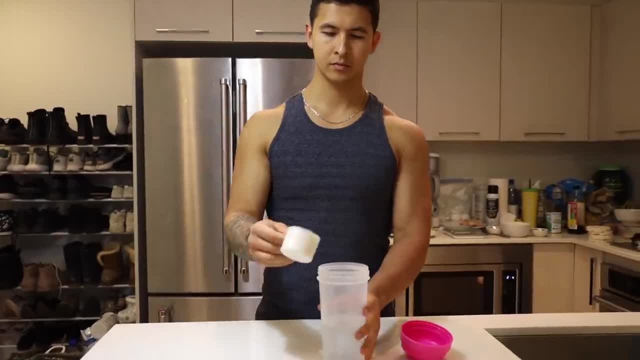 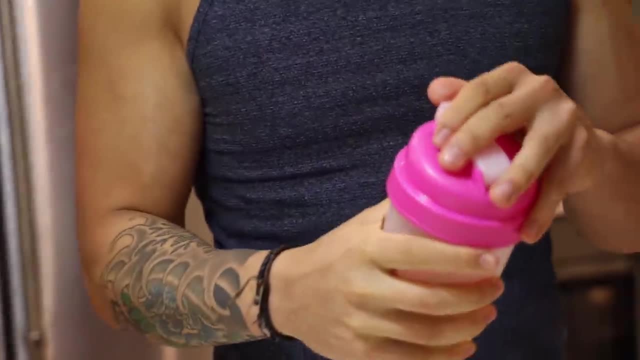 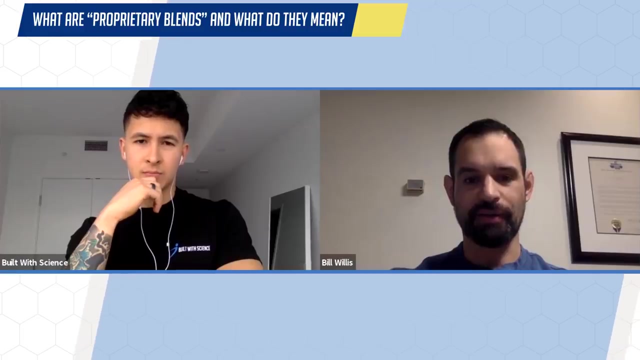 Sure, yeah, that's something you have to watch out for with any protein product. The issue is that most whey proteins in particular are made of isolates and concentrates generally, sometimes some protein hydrolysates, And what you'll find is, you know, a proprietary blend on the listing label and in this blend. 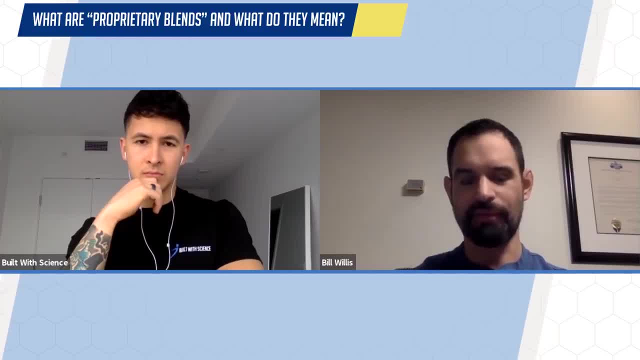 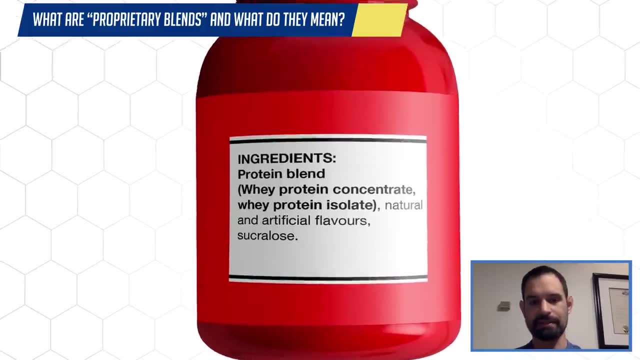 the company doesn't really have to disclose the amount of anything that's in that blend. So, for instance, if you look at the back of a label of whey protein powder and it's a blend of whey concentrate and isolate, you know that's great. 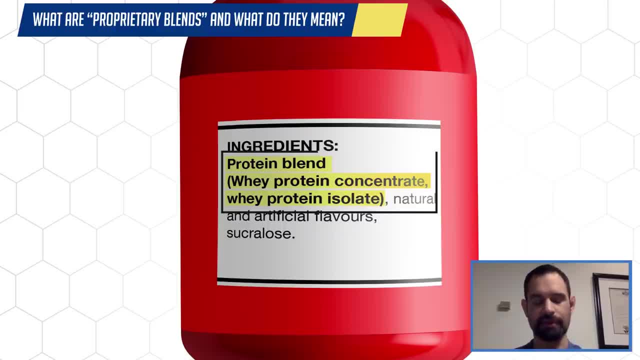 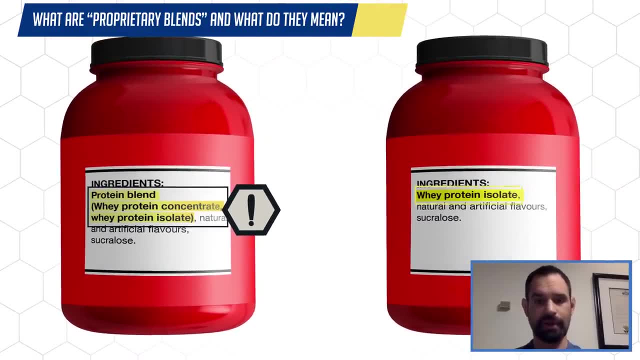 Concentrate can be good, an effective source of protein, as can isolate. But the issue is is that the concentrate could be a really cheap, low quality one And there could be just a tiny little trace amount of isolate. So in that example, let's say, you, an unscrupulous manufacturer, put a proprietary blend in there. 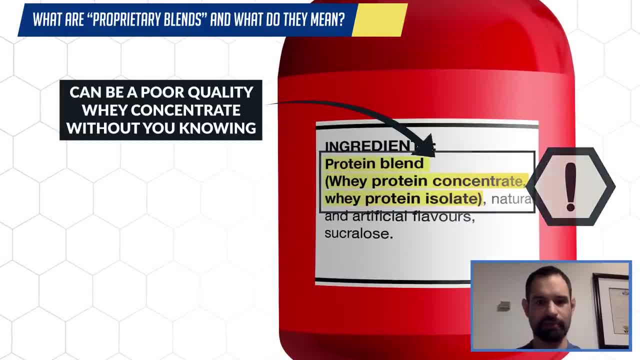 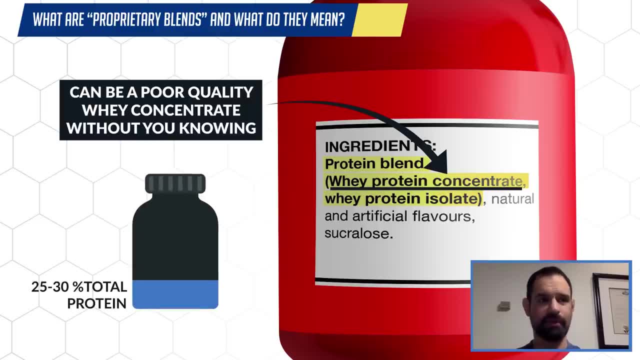 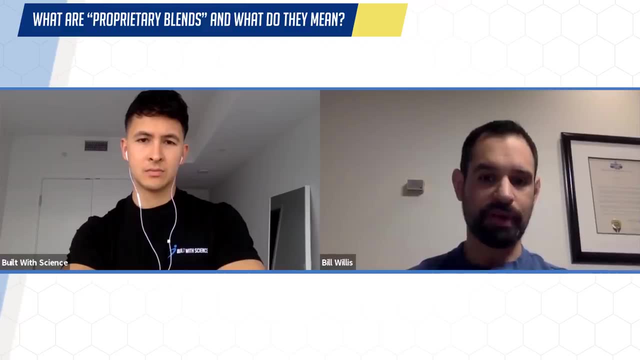 Because they got a delivery of some really cheap whey concentrate that they got for a good price. that was low quality. In this case, that whey concentrate could be, you know, as low as 25 or 30% total protein. Now the claims on the label in terms of the total protein content may be met with that. 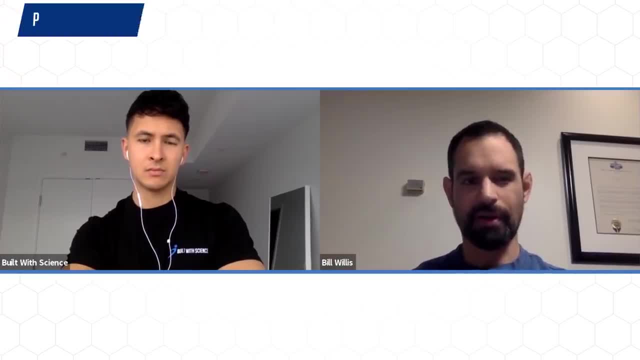 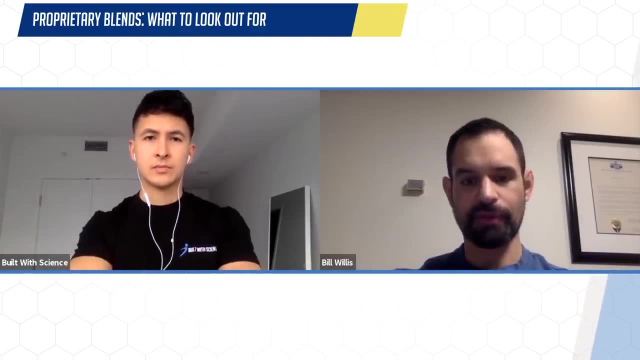 blend. You know, everything might be on the up and up there, But what you can look out for is the serving size, In particular, How much protein is present per serving relative to the serving size. So you take a look at the label and let's say you're you know you're dealing with. 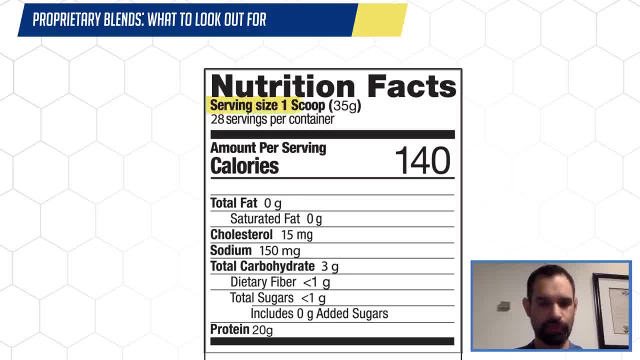 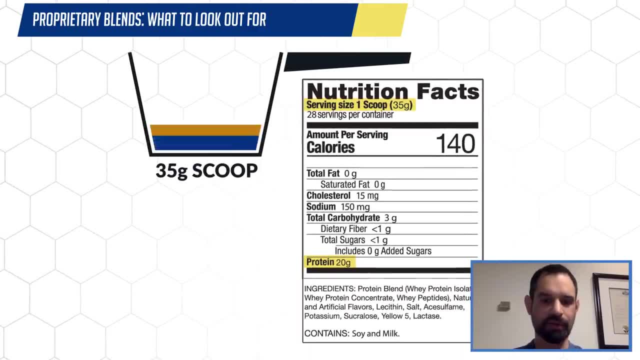 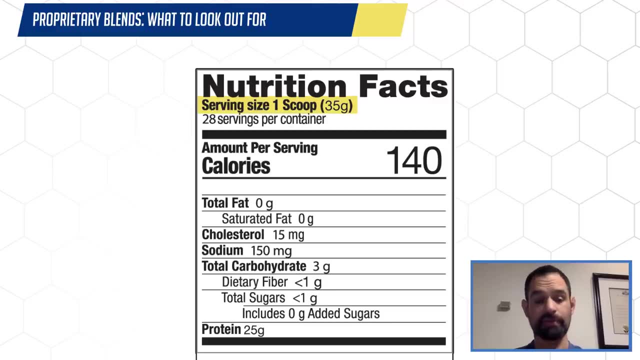 whey protein And product A is in a 35 gram total serving. let's say there's 20 grams of total protein. That's going to be relatively low, indicating a lower quality protein. On the other hand, let's say, for that same 35 gram serving size, another type of whey. 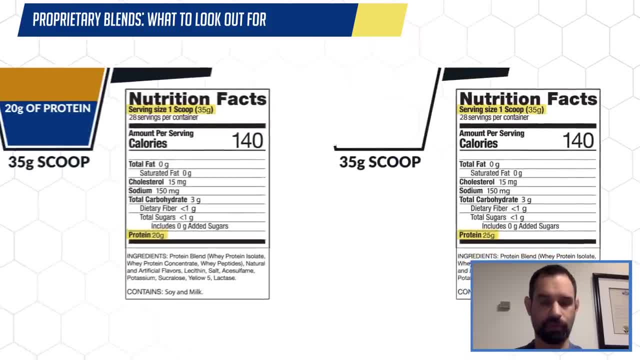 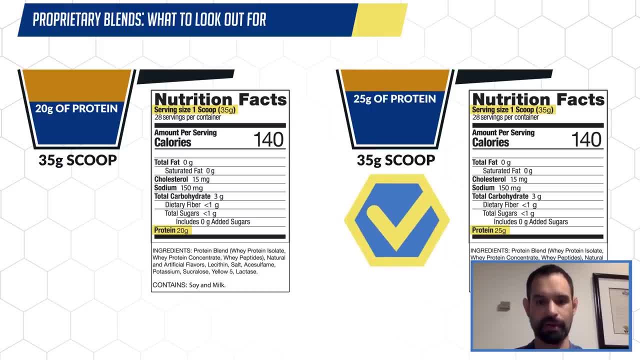 has maybe 25.. Or even up to 28 grams in that total 35 gram serving size. That one would be higher quality and that's what you want to look out for. You want to get the protein with the most total protein per serving. 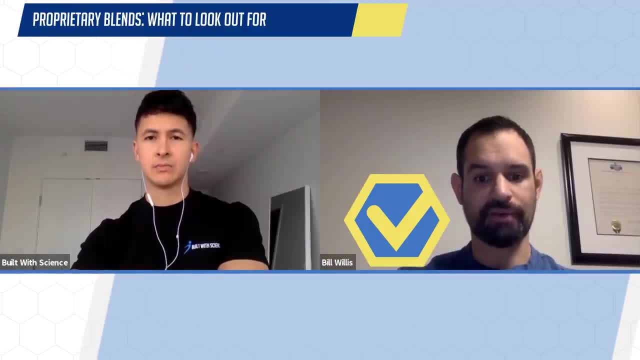 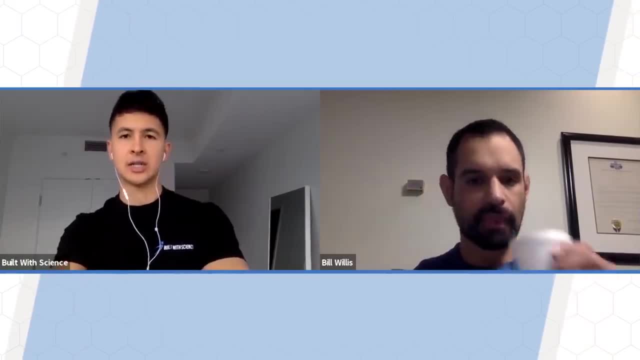 Those proteins are higher purity. Otherwise, you'll be paying for less of what you really need in a protein and more of just the junk in the fillers. As far as I know, even if we do look at the protein content on the back of the label, 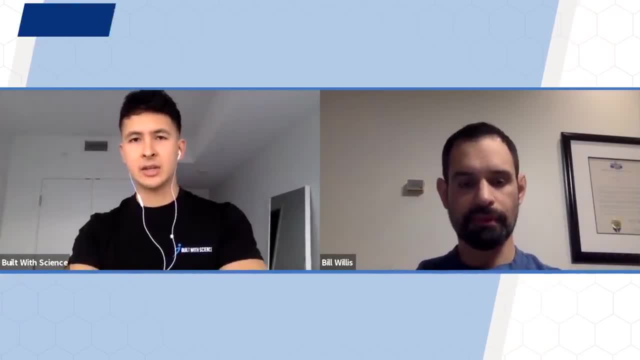 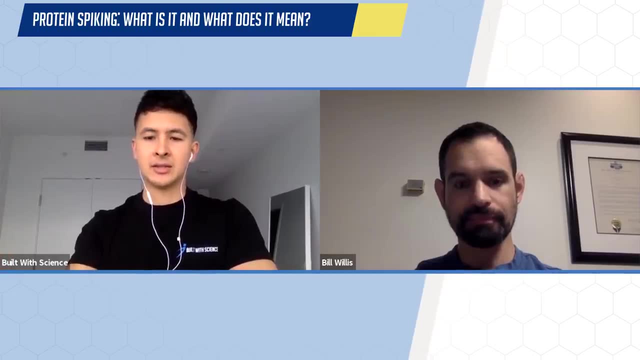 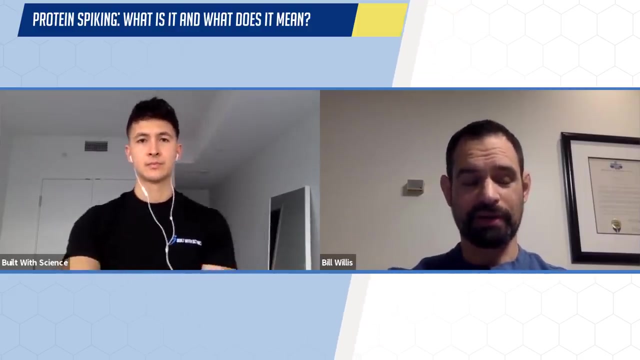 there's still A loophole that companies can actually use to deceive us, And it's with something that's called protein spiking. What exactly is protein spiking? and, again, how can us, as consumers, avoid falling into this trap? Yeah, that's a. that's a dirty trick. 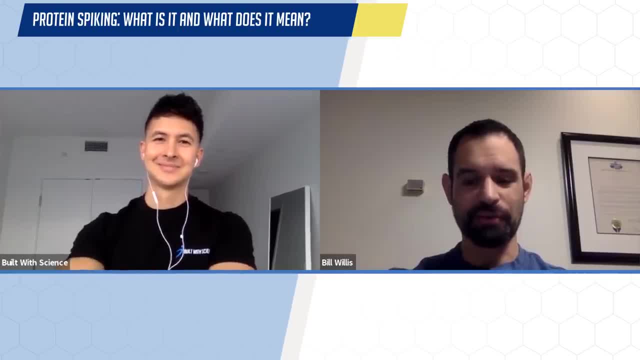 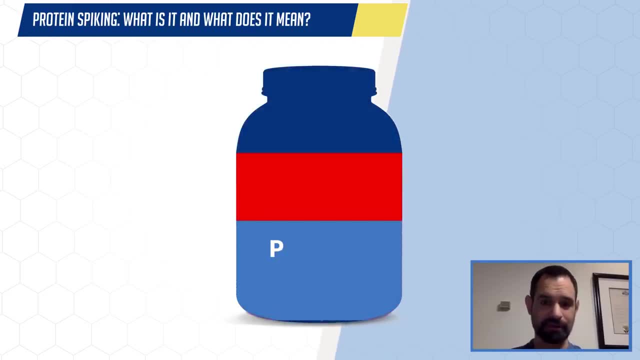 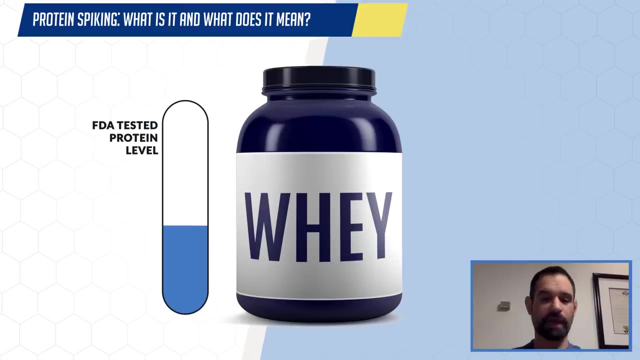 And how dirty it is, I guess, depends on what exactly they do. So protein spiking is adding a non-protein nitrogen containing substances to the protein powder that will be measured as protein, And the thing is that the FDA tests just total nitrogen levels and it's a quick and dirty. 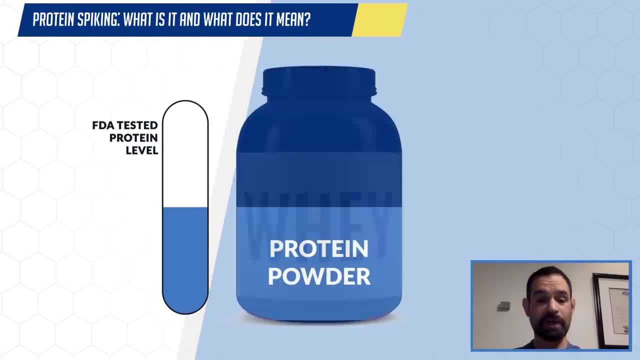 way to assess protein content. Now the manufacturer could add extra nitrogen containing agents in there that aren't protein- Creatine is commonly used- or maybe a cheap free form amino acid such as glutamine, And again you'll see this in like a proprietary blend. 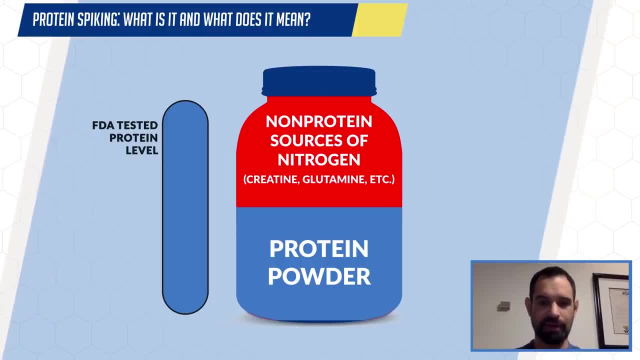 You might see whey isolate, whey concentrate, Yeah, Even glutamine. Well, you know, you don't know exactly how much of which is in there. and that's when they do it legally. When they do it in illegally, they're just going to throw any extra nitrogen containing. 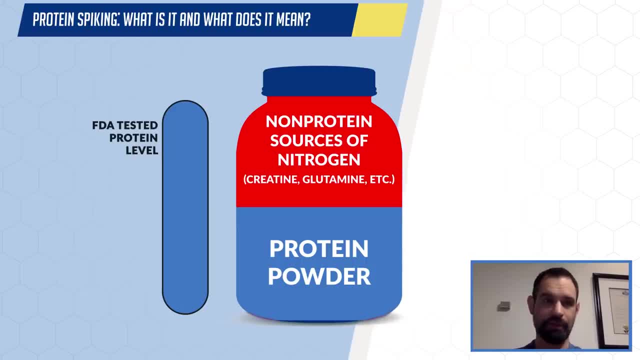 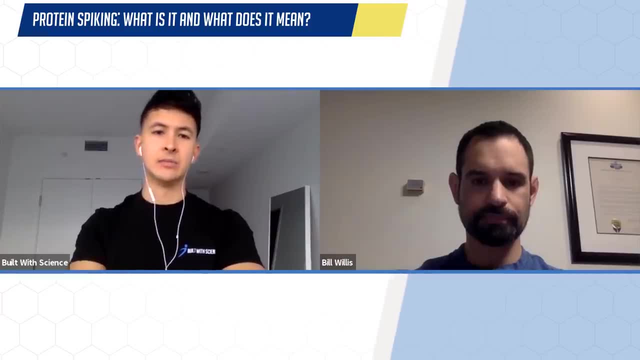 substance in there and it's not going to be stated on the label. The latter is, as I mentioned, just a little sneakier and it's a little harder to detect. I guess, again, what you could also do is just look at the ingredients label and avoid. 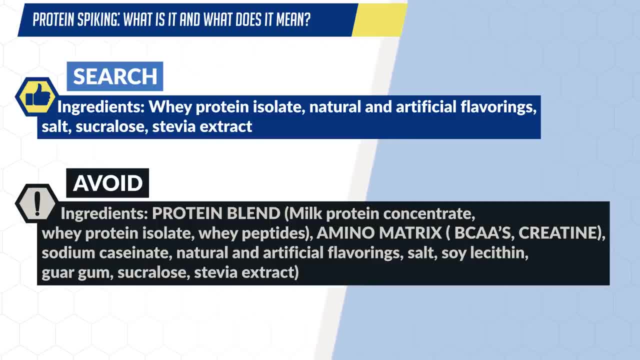 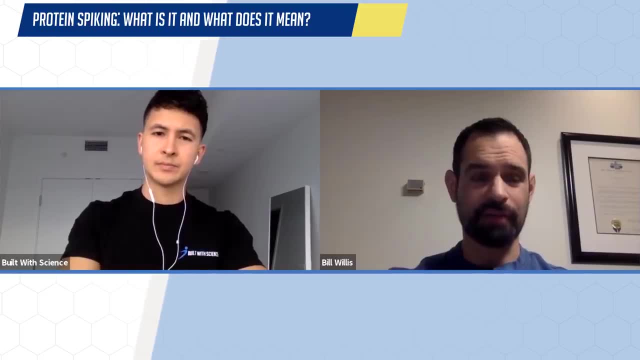 protein blends Avoid- I mean you mentioned amino acids, glutamine or amino acid matrix matrices or amino acid blends- as those are potential indications that the protein has actually been spiked. Yeah, Yeah, Actually, you have to watch for that, because a lot of times these proprietary blends are. 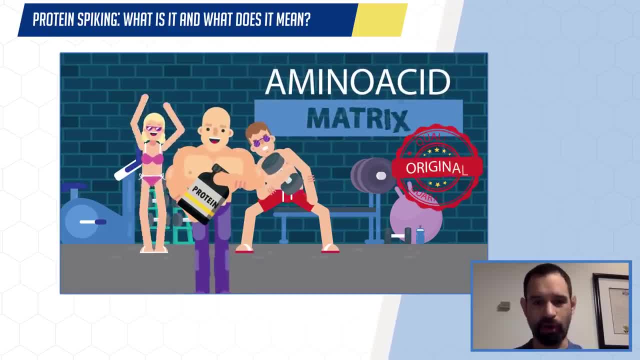 especially like the amino acid matrix, will show up in their marketing. Like you'll be thumbing through a fitness magazine and you'll see this big, bright, shiny bottle of protein And you know, these superhero looking like people that are, you know, supposedly got. 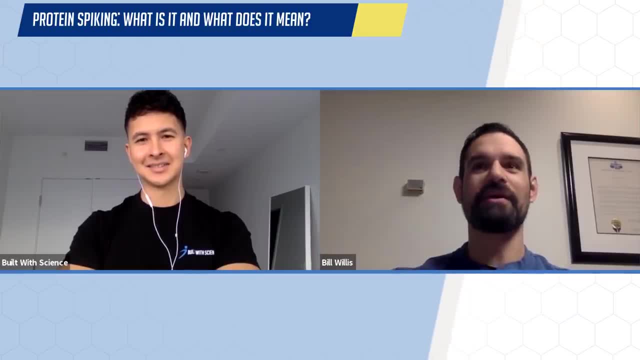 their physique that way, and you know proprietary amino acid matrix They sort of use that It's hidden in plain sight. in a way, The consumer links- you know this, this fancy term- to the physique of the you know whoever. 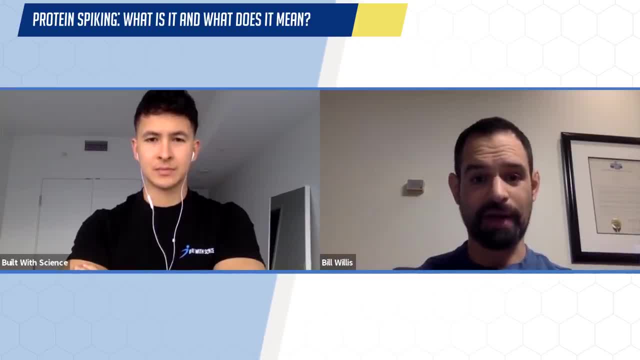 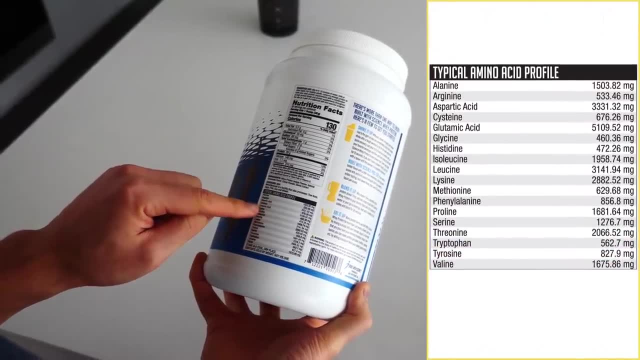 they're getting to endorse the product And really that's where they're hiding. you know the lack of protein quality on the label, So you really have to watch out for that. Look for brands that fully disclose the amount of amino acid or the amino acid profile, rather. 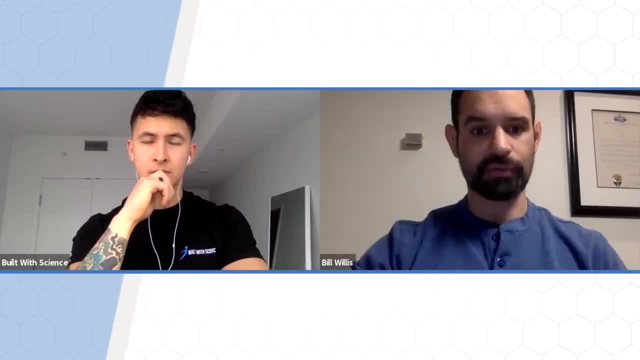 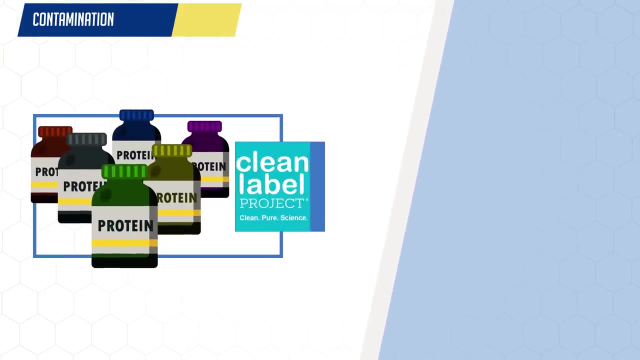 of their protein. This helps indicate that they're fully transparent about the specific amino acid content of their product and are less likely to have spiked it. The last and final thing to look out for is contamination. Third party testing. results from a 2018 analysis by the Clean Label Project found that among 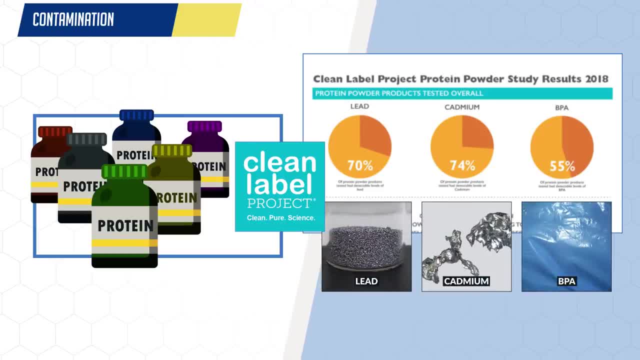 a hundred and thirty four Tested protein powders. the vast majority of them had detectable levels of heavy metals and plastic derivatives as a result of their ingredient sourcing and manufacturing practices. Now, detectable does not mean dangerous, but many of these protein powders did indeed have. 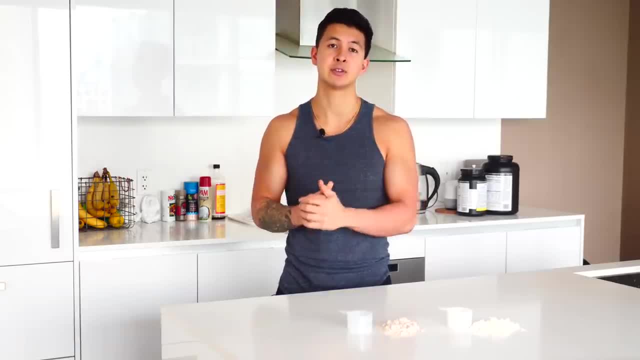 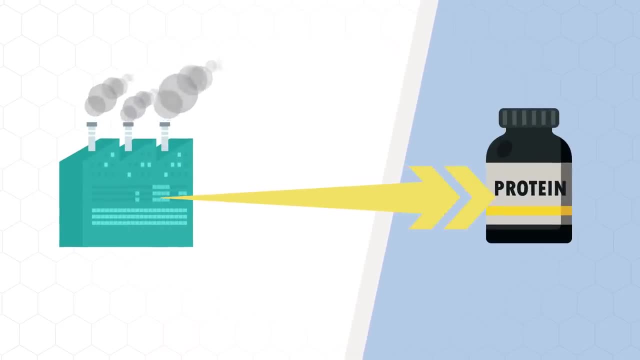 levels that surpass the acceptable levels, which is something you'd obviously want to avoid. And this is a common occurrence because supplement companies aren't required to test their products for contaminants and are instead left voluntarily to run those tests. So, to minimize your risk as a consumer, simply do a little bit of digging around to see.